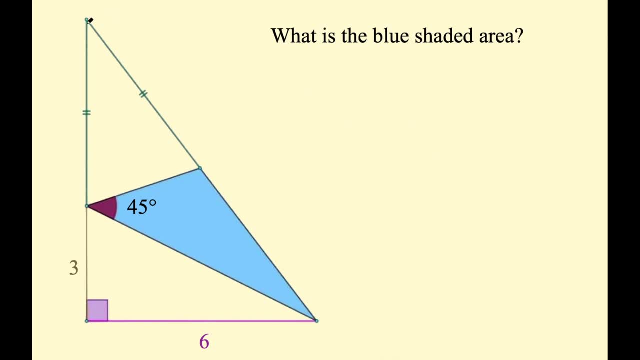 plane geometry. Okay, so this first question gives us a right triangle, and then in the corner there's an isosceles triangle. We're looking for this blue shaded region. All they tell us is: this angle is 45 degrees, this length is 3, and this length is 6.. A reminder to pause the video now. 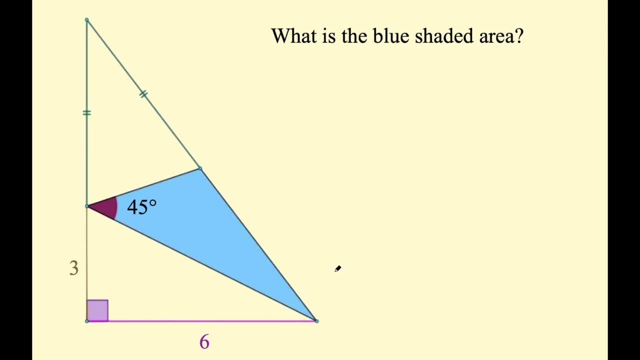 if you want to give this problem a go yourself To solve this. we're going to go on a bit of an angular journey looking at the angles throughout this diagram, and I'm going to start here. I'm going to label this angle theta. Then this angle up here is 90 tate theta. This angle in here. 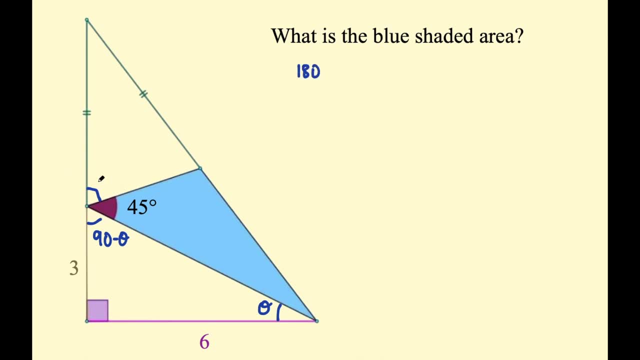 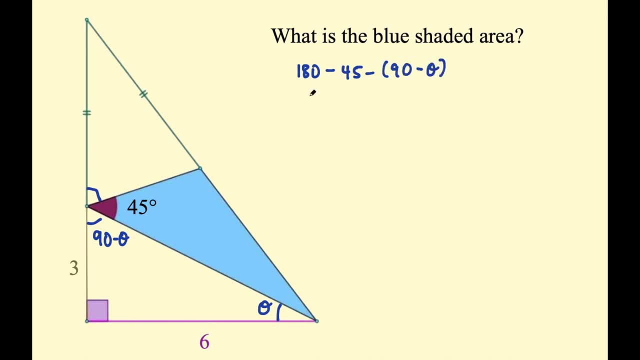 subtract 90 tate theta. What's this? Well, this is 180, tate 90 is 90,, tate 45 is 45, then subtract negative theta is positive theta. So this angle in here is 45 plus theta, and because this is an 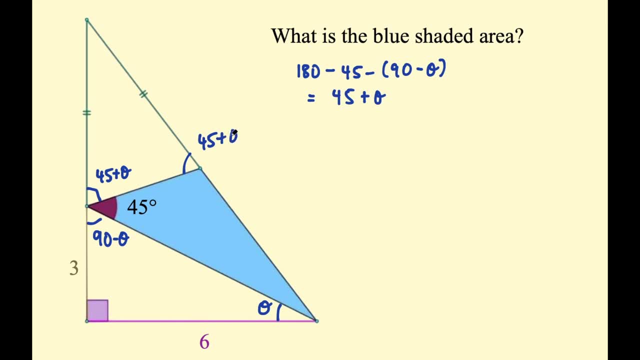 isosceles triangle. this angle will also be 45 plus theta. Going to pause there on the angle hunt for a minute, Going to look at this area. Well, we can work out the hypotenuse. We'll do that in a 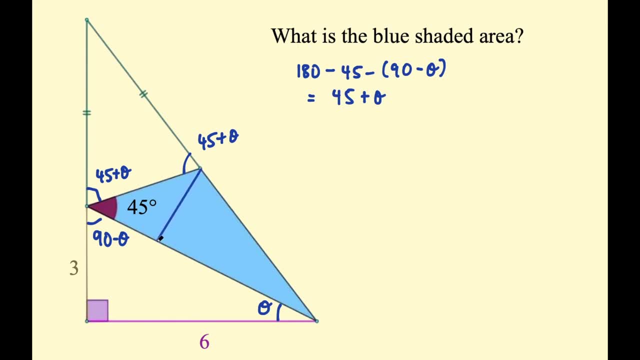 minute. But to find the area, we would like to know the perpendicular height So we can draw a line perpendicular to the base here, joining up to this angle. Then what we've created is a 45,, 45, 90 right triangle. Okay, so this angle in here is 45. Let's find this angle. That's going. 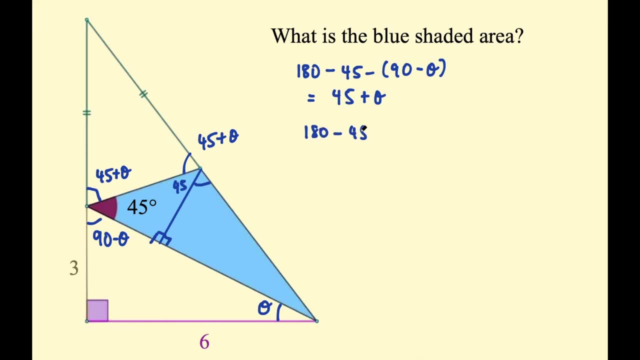 to be 180, take 45,. take 45 plus theta. So this is 180, take 45,. take 45 plus theta. So this is 180, take 90, that's 90, subtract theta. Okay, so this angle in here is 90, take theta. That means 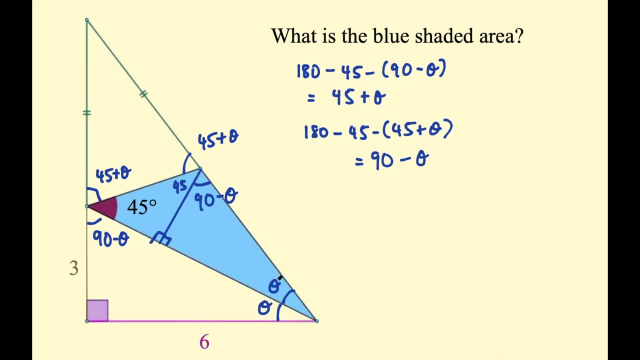 this angle over here must be theta. So I did all of that to find that this larger angle is bisected by this line. There might be an easier way to show that. at least that's how I did it. Okay, so now these two right triangles are similar and I'm going to go ahead and find 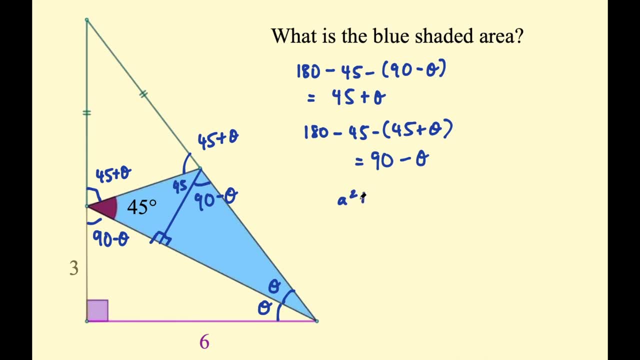 the hypotenuse now. So, using Pythagoras' theorem, a squared plus b squared equals c squared. c squared is going to be 3 squared plus 6. squared 36 plus 9 is 45.. So c is equal to the square root. 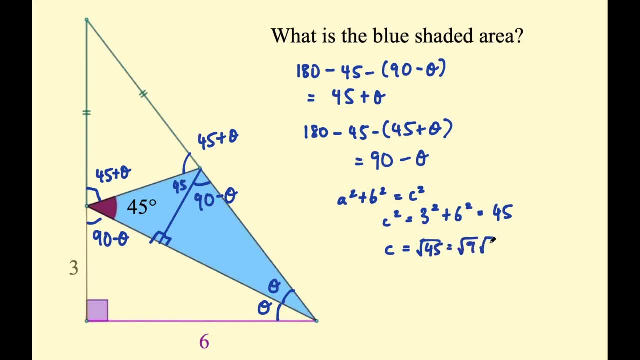 of 45,, or the square root of 9 times the square root of 5, or 3 root 5.. Okay, so that's the length of that hypotenuse. Let's just write that down there. That's that. 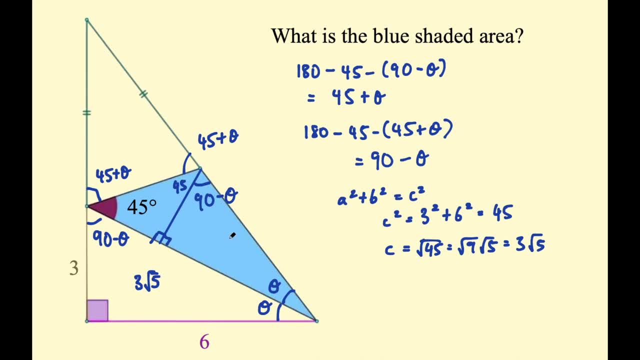 Length. And now let's have a look at this blue triangle, focusing on this right triangle that's similar to this larger one. Well, these sides are in the ratio 1 to 2, 3 to 6 is the same as ratio. 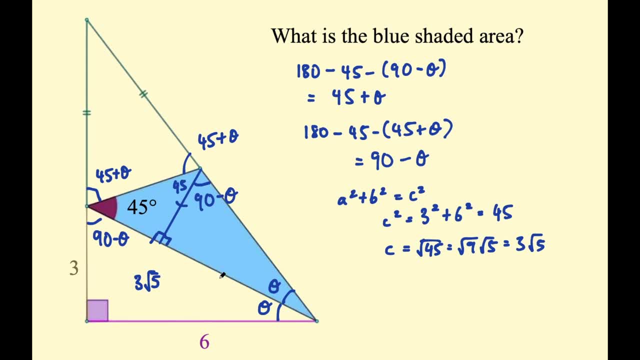 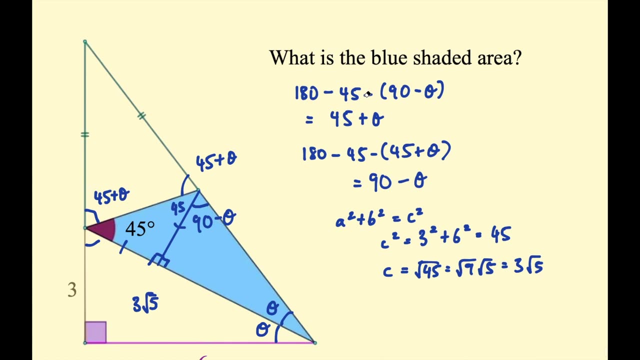 1 to 2.. So these lengths must be in the ratio 1 to 2.. These two lengths are equal. In any 45-45-90 triangle the two legs are equal. So let's get rid of this For a second. So if, if, excuse me, if- these two legs are in the ratio 1 to 2, then these two legs 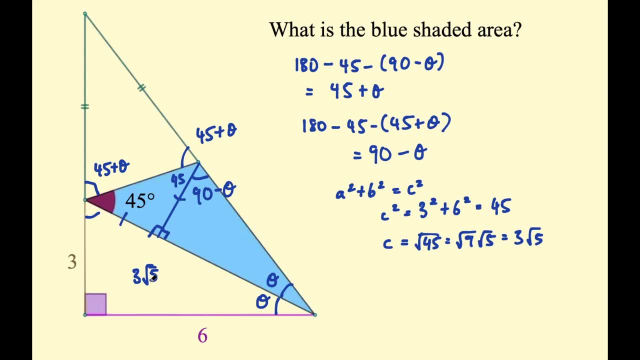 must be in the ratio 1 to 2.. We know the entire length is 3 root 5.. So this part of that length must be one lot of root 5.. This length here must be two lots of root 5.. Okay, why did I do that? 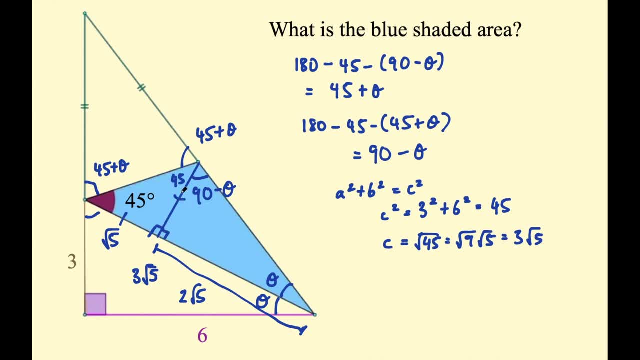 Well, that means that if these two legs are equal, this length in here- let's get rid of some of this- This length in here must also be root 5.. Okay, now we have that perpendicular height, We have the base, We can work out the area. 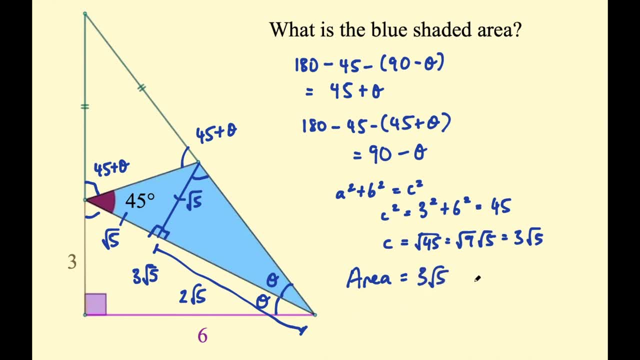 The area is going to be the base: 3 root 5 multiplied by the height divided by 2.. So 3 root 5 times root 5 is 15.. It's going to be 15 on 2 or 7.5.. There we go. That's the. 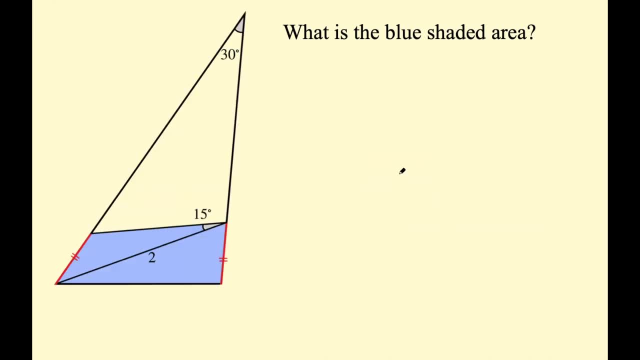 area of that blue triangle. Moving on to the next problem, then Again we're looking for a blue shaded area. This one's a little bit harder than the last one. I started this problem by working on a special case. I began by assuming this triangle was an isosceles triangle. It didn't. 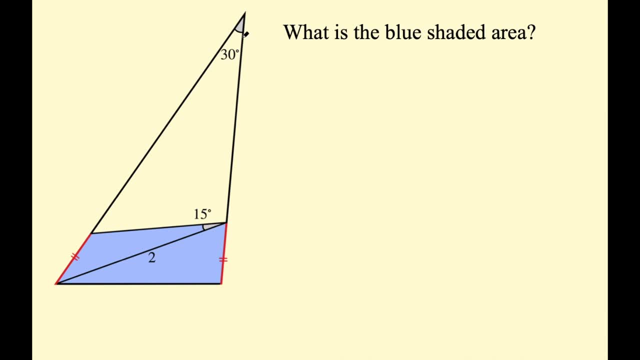 really help me to prove the general case, though, So we'll talk a bit more about that at the end. So let's go ahead and see if we can prove or find this area in general for any triangle with these properties. So all we're told is: this angle is: 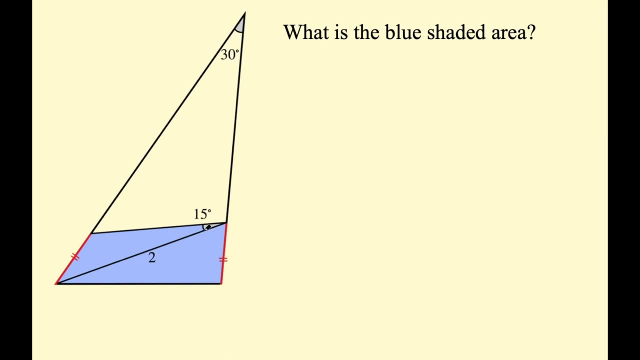 degrees. this little angle angle in here is 15 degrees and this line has a length of two. these two lines are the length of those. two lines are equal. again, if you want to give this problem a go, pause the video now. okay, where to start? you can really start anywhere. i began by labeling this: 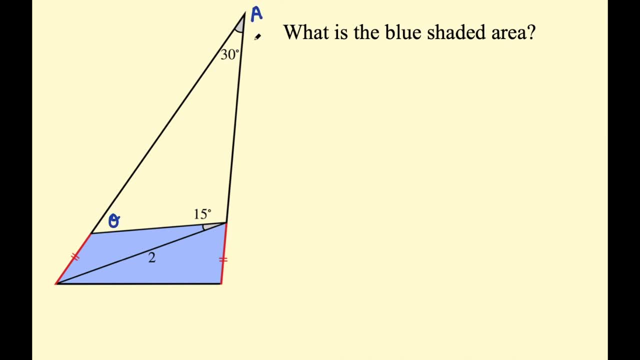 angle, theta, and actually let's give these points labels as well, say a, b, c, d and e. so angle a, b, e, a, b, c. sorry, let's say let's call that theta. then therefore, angle a, c, b equals 150. take theta, the sum of these two angles must add up to 150. then angle d, c, e is this one in here. that's going. 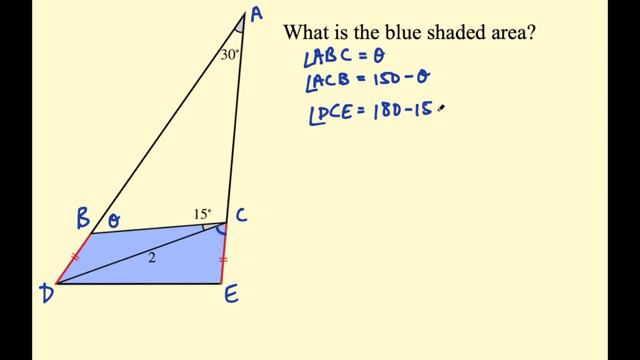 to be 180, take 15, take 150, take theta. okay, what's this? well, this is 180, take 150 is 30, take 15 is 15. subtract negative theta is plus theta. when i was trying to work this out at this point, i still didn't have a general strategy on. 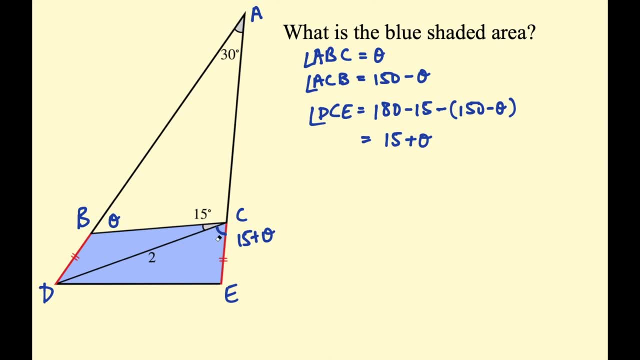 how to solve it. but i found this interesting. so what i did next was to split this angle into 15 degrees and theta degrees, because why not? so i'm going to call this angle in here 15 and this angle is theta. okay, oops, and what next? well, often in geometric problems where you're told two lengths are the, 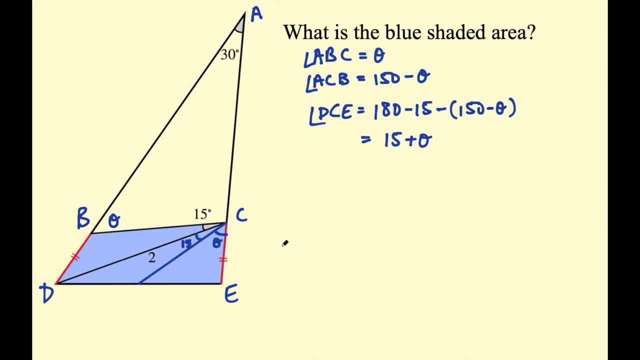 same. it's often a good strategy to try to relate them somehow, so, you know, get them close together or draw some construction that relates those two lengths, um, maybe in the same shape or in the same triangle, somehow. so what i tried next was to extend this line cb. 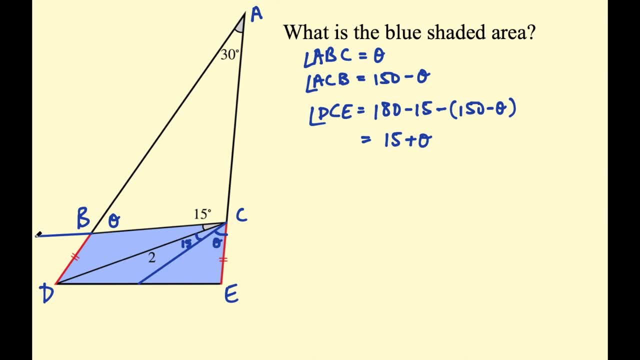 so, straight out this way, and because these two lines are straight, these angles are vertically opposite. therefore, this angle is theta. so now what i could do is i could create a congruent triangle to this triangle in here. let's label this point m, c, m, e, because, um, this angle is theta. 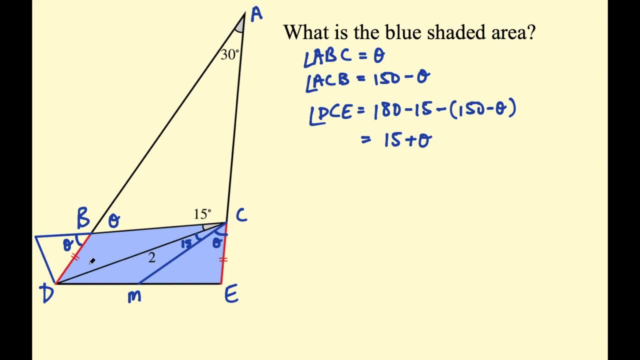 and it's adjacent to the same length. i could construct a congruent triangle over here, but from there i'm not sure how to proceed. so the next thing i tried, still with no clear idea of of a strategy, i tried constructing a 90 degree angle here, because right triangles have really nice properties. 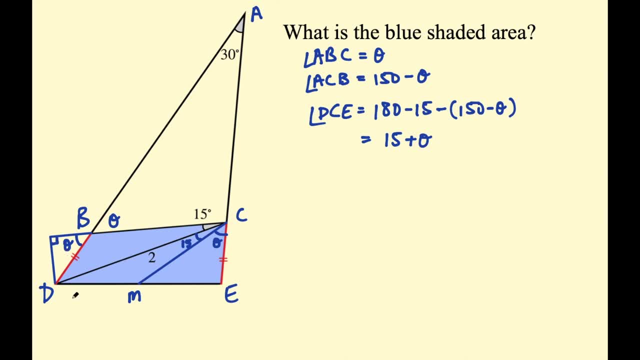 and often it's really useful to use right triangles in solving areas. so i created a right triangle here. it has an angle of 15, a hypotenuse of 2 and well, this triangle doesn't seem to have anything to do with this triangle, cme, but if i draw a line perpendicular to cm, so this is 90 degrees. 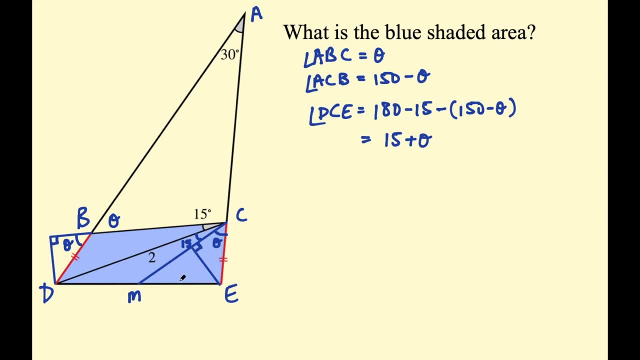 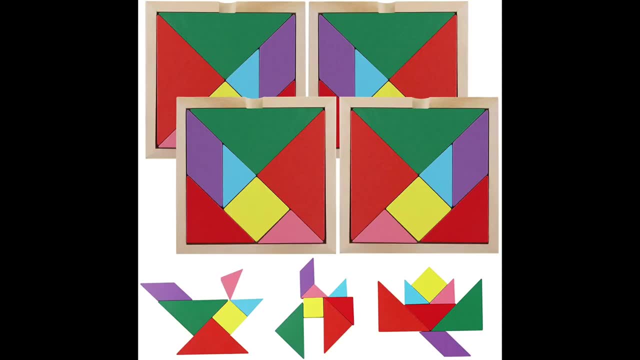 then these two triangles are congruent. and now we're kind of trying to play a game of tangrams. do you remember that tangram game where you had all the pieces and you tried to make shapes out of them? that's what we're sort of trying to do here. we're building a 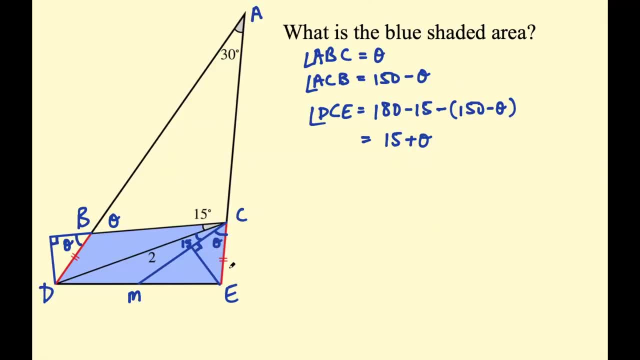 we're playing a bit of a jigsaw puzzle, and the strategy now is, rather than looking for these perpendicular heights, is to try to rearrange these pieces into a shape that i can easily find the area of and i'm already. i have already taken this part. 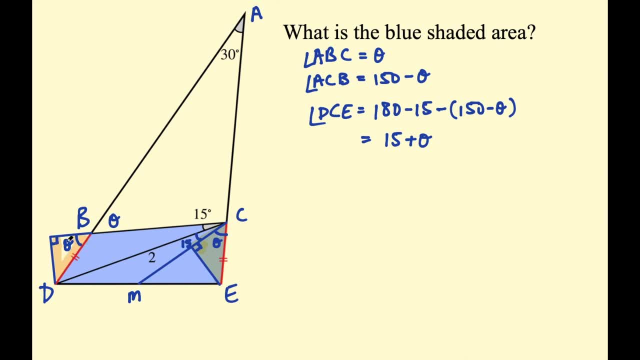 and created a nice right triangle. i don't know the height of this right triangle, but i do know that. do know the hypotenuse and one angle in that right triangle. okay, next, this is the hardest step that i found, um, and i'm not sure how to suggest seeing how to do this other than 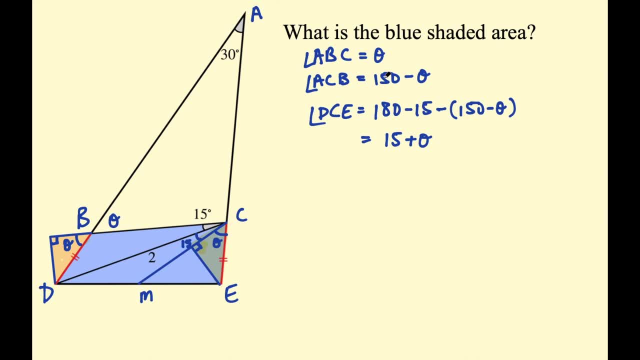 through pure experimentation and messing around. what i tried next was to extend this line c, m and construct another right triangle. okay, so again, this is a right triangle and i just want the left triangle needed. so here that is the left triangle, that's my left triangle, angle 15, hypotenuse 2, and actually it must be congruent to the other right triangle. let's label: 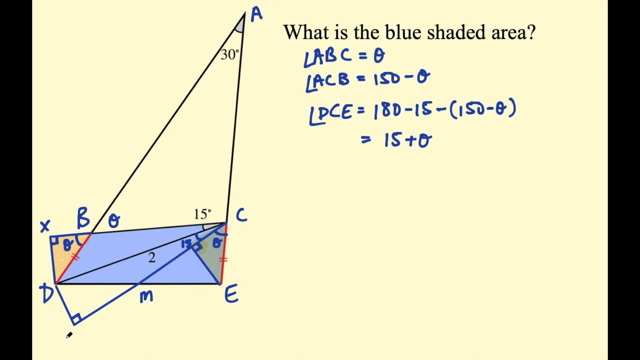 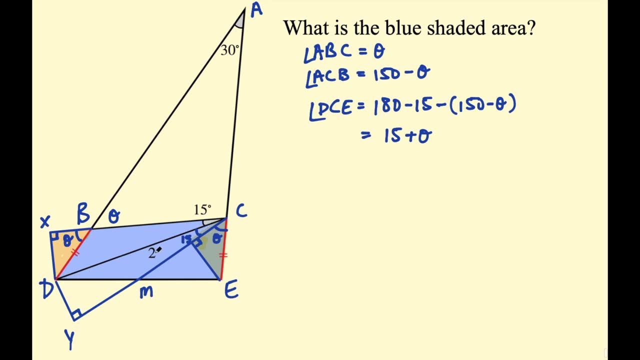 this point x. so, and actually let's label this one y. so cyd must be congruent to cxd. this is the angle angle side rule of congruence: two angles and a side the same. therefore the um, the triangles, are the same. uh, they are congruent. so now i know that they're congruent. is there anything i can say? 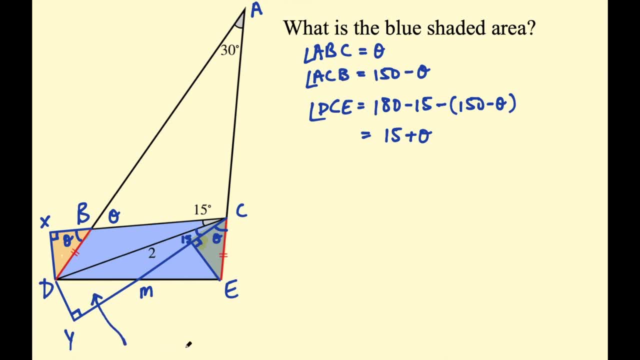 about this right triangle in here. is there anything helpful i can say about that right triangle? uh, this little one, dmy. well i know this length must be the same as xd. dy must be the same as xd. again, they're congruent triangles. all of the legs are the same length. these two angles are vertically. 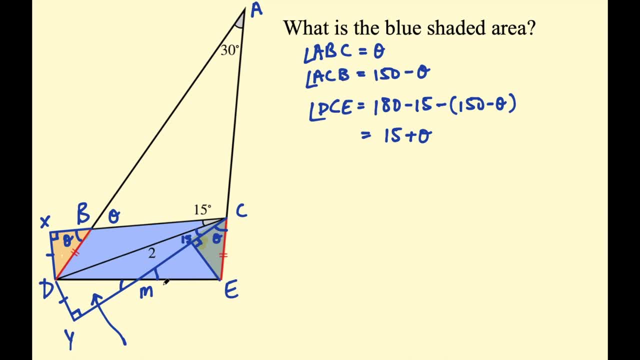 opposite. therefore they're equal. and what else? well, what is this leg in relation to this triangle over here? this leg xd relates to this leg, so these three lengths are the same. this was a 90 degree angle. this was the most surprising part of this problem for me: finding that these two right triangles are 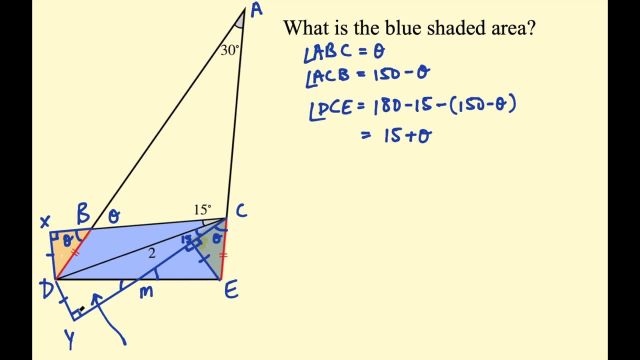 also congruent, again using that angle angle side rule of congruence. so again we've played the jigsaw game where we have taken this right triangle and shifted it over here. i was really surprised by this. i am still not sure i 100, 100 understand. 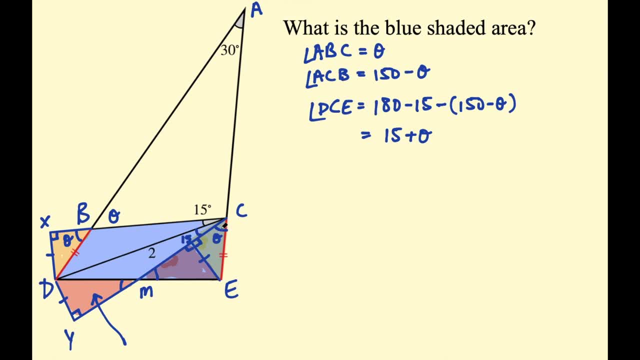 this problem. it also means, by the way, if you notice, that this line must bisect de and again i. i feel like there's a deeper reason behind that, but i'm not sure what it is. so, anyways, we've rearranged the jigsaw puzzle, we've taken these two pieces and created two jigsaw pieces, and we've 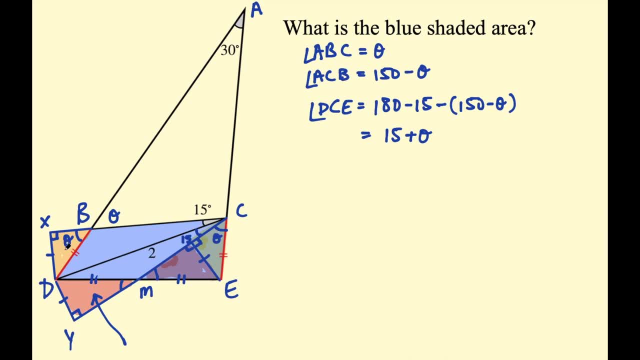 taken these two pieces and created two jigsaw pieces, and created two jigsaw pieces and created two congruent right triangles, and those two congruent right triangles contain the area, the original blue area. we've just shifted around the pieces. so then, to find the blue area, let's 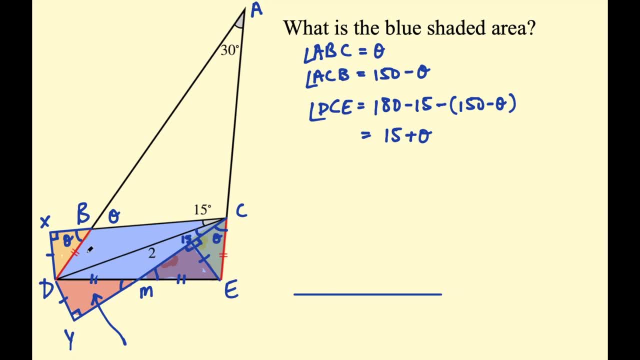 draw another diagram over here. so here i'm going to draw one of the right triangles with the hypotenuse as the base, so this is a 90 degree angle. then i'm going to stack the other right triangle on top of it, such that the two right triangles are the same as the base. so this is a 90 degree angle. then i'm going to stack the other right triangle on top of it, such that the two right triangles are the same as the base. so this is a 90 degree angle. then i'm going to stack the other right triangle on top of it, such that the two right triangles are the same as the base. so this is a 90 degree angle. then i'm going to stack the other right triangle on top of it, such that the two 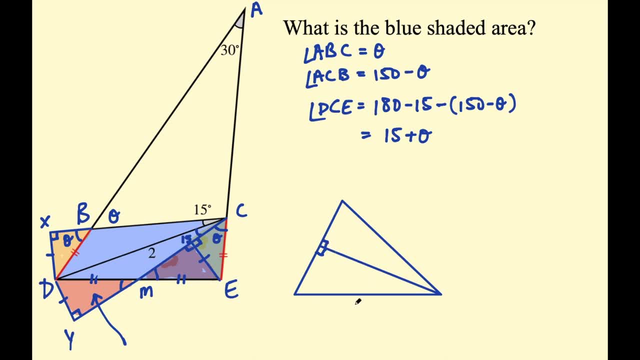 identical legs are together, so this length is two. both of them had angles of 15 degrees, which means this total angle is 30 degrees. and then let's drop a line perpendicular. and then let's drop a line perpendicular to the base, so that will be the perpendicular height. 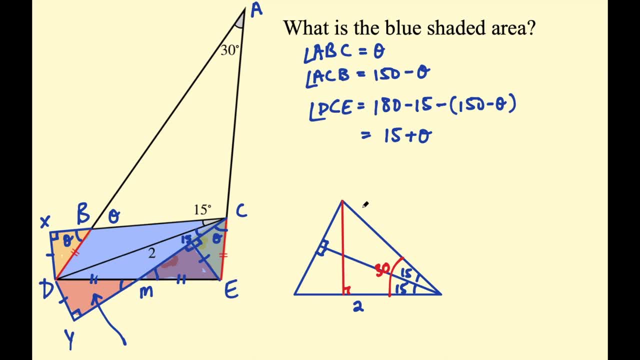 of this larger triangle and, lastly, we notice this hypotenuse. so this has a length of two. so this has a length of two. here we have a. here we have a. here we have a 30, 60, 90 right triangle with hypotenuse of. 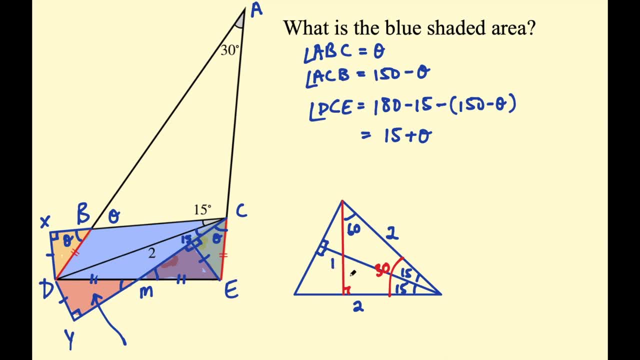 30- 60- 90 right triangle with hypotenuse of 30- 60- 90 right triangle with hypotenuse of two: two, two. that means this leg must have a length. that means this leg must have a length. that means this leg must have a length of one. see my video on exact values for. 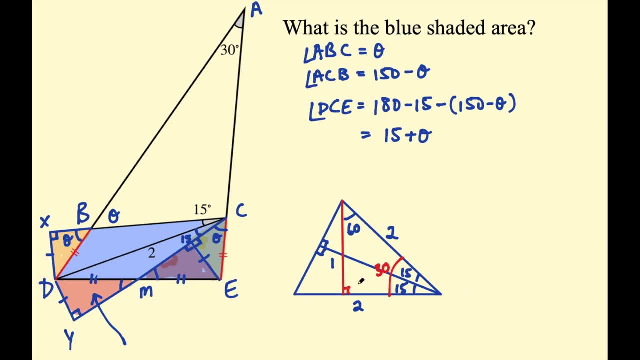 of one- see my video on exact values for of one. see my video on exact values for more detail on that, more detail on that, more detail on that. then we have a base of two perpendicular. then we have a base of two perpendicular. then we have a base of two perpendicular height of one. 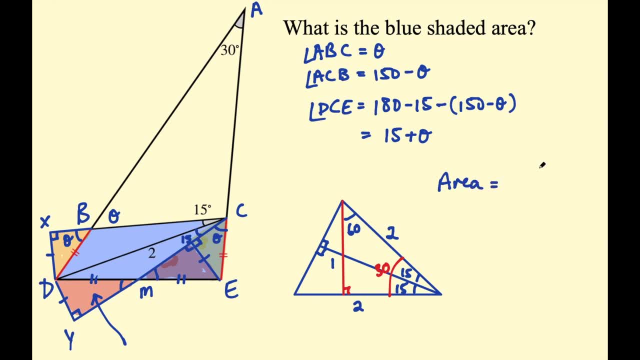 height of one, height of one. we have enough to find the area that's. we have enough to find the area that's. we have enough to find the area that's going to be base, going to be base, going to be base times height divided by two, which is 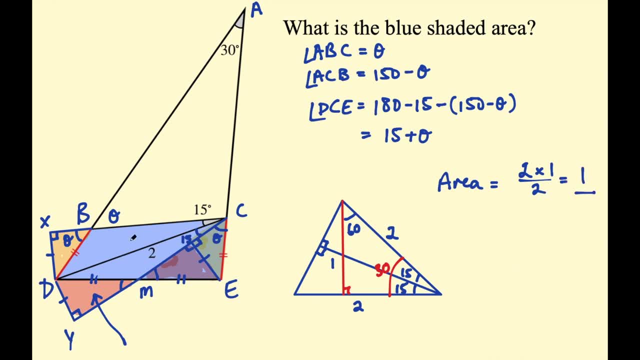 times height divided by two, which is times height divided by two, which is two, divided by two, which is one. two divided by two, which is one. two divided by two, which is one, so that blue area has an area of one, so that blue area has an area of one. 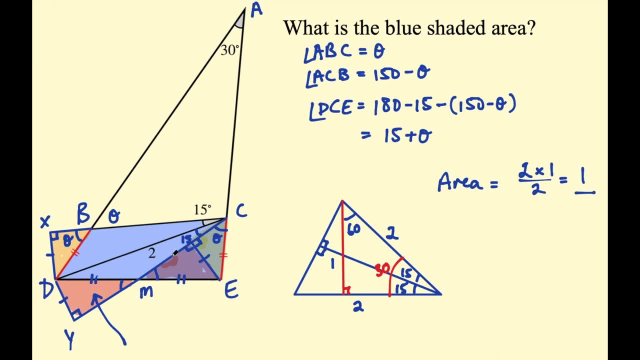 so that blue area has an area of one unit squared, whatever the units are unit squared, whatever the units are unit squared, whatever the units are pretty nice right? let me know what you pretty nice right? let me know what you pretty nice right? let me know what you thought of those problems. please leave a. 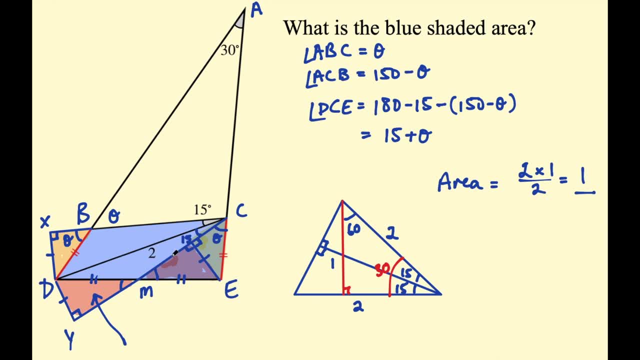 thought of those problems. please leave a thought of those problems. please leave a like if you appreciate this video. like if you appreciate this video. like if you appreciate this video. subscribe if you want to see more subscribe if you want to see more subscribe, if you want to see more content. and i'll see in the next one. content and i'll see in the next one. content and i'll see in the next one. bye for now.